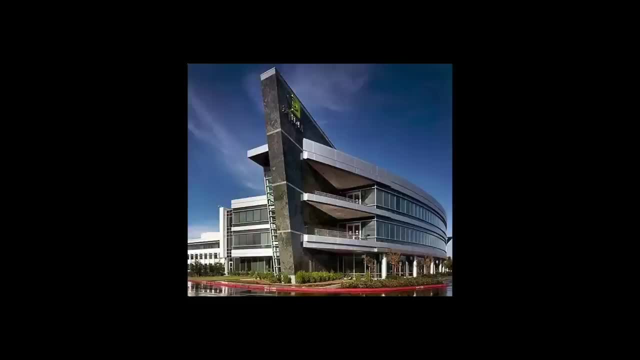 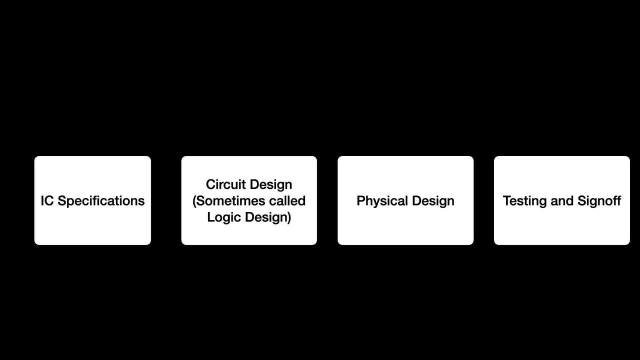 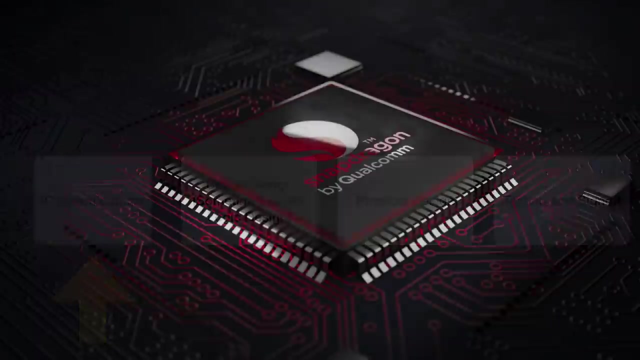 How does a company like Apple or Nvidia design their custom chips? The process and the names might differ from company to company, But a generic flow might look something like this: First, the product designers and system engineers at a high level envision a product They might not know too much about: circuit design. 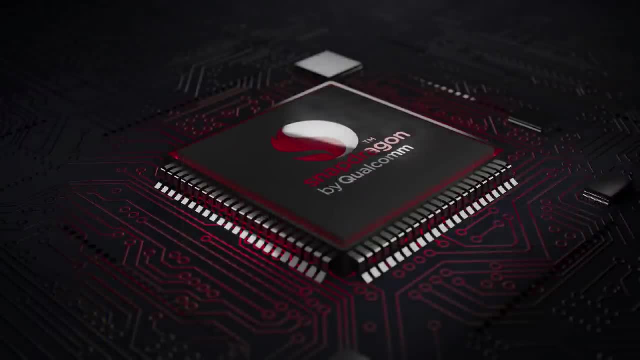 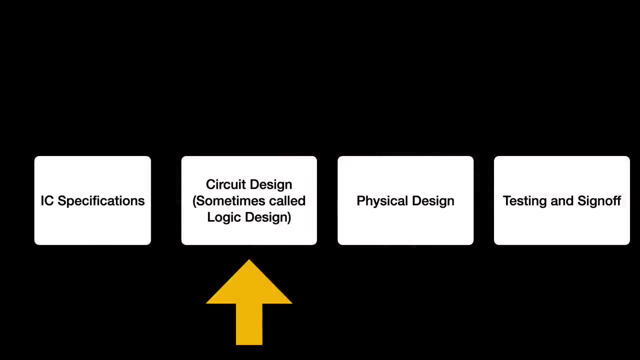 but they do know what their customers want, And so they come up with a set of integrated circuit requirements based on the customer's needs. Next, the chip's requirements enter logic design, also called circuit design. These people translate abstract requirements into circuits with the logic capable of meeting those requirements. 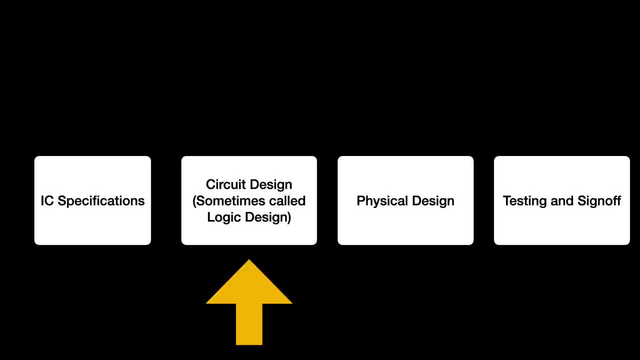 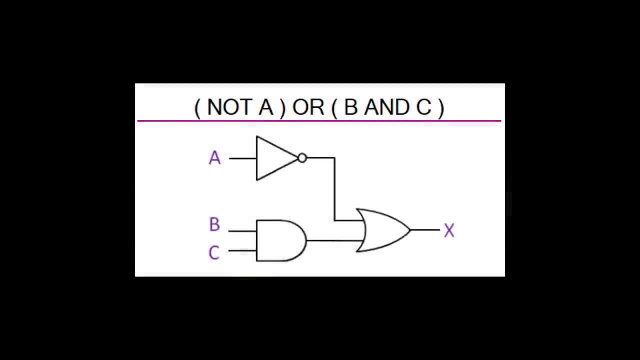 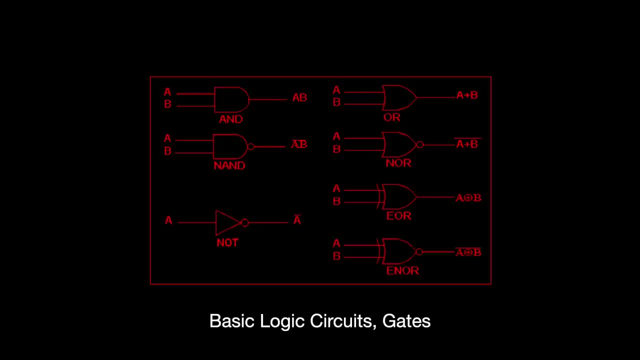 Think of it like a UX designer who crafts how a software feature might look, act and feel together with a product. A chip has many circuit designs on it and those circuits do different things. I'll briefly touch on two such circuits. Logic circuits or gates act sort of like a decision box. It receives inputs. 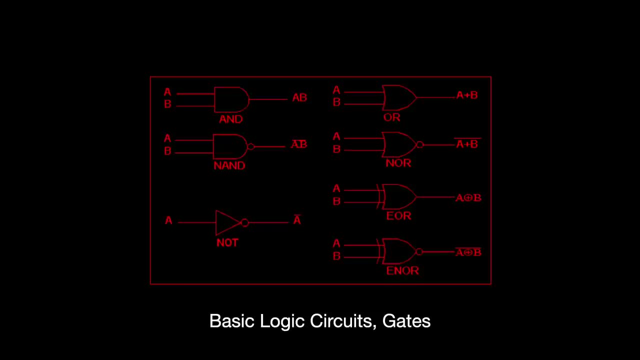 puts them together and comes out with an output: Is A equal to B? D is true only if E and F are also true. Stuff like that, Just one logic circuit by itself, can seem pretty simple, but in groups they can do amazing things, Like zombies. 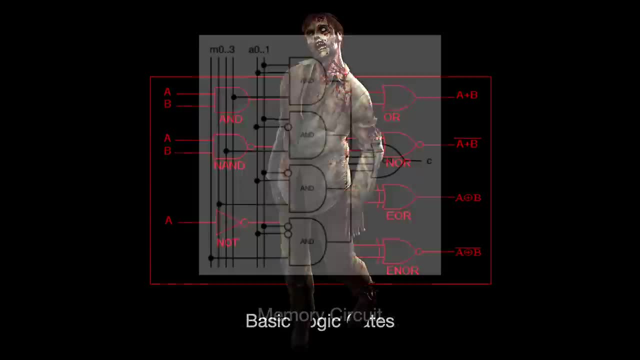 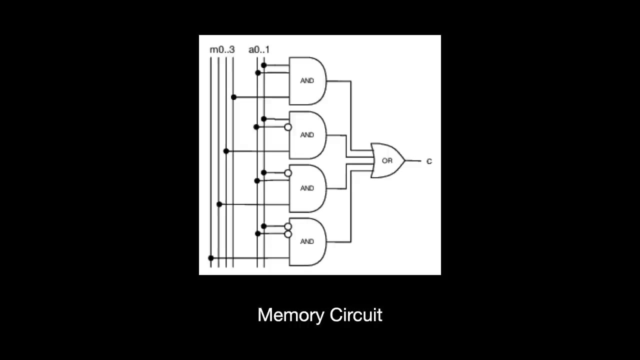 The second type circuit is called a memory circuit. It is capable of remembering whether a value was true or false, Kind of like a light switch that is on or off. Once the logic designer has completed their work, they end up with groupings of logic and 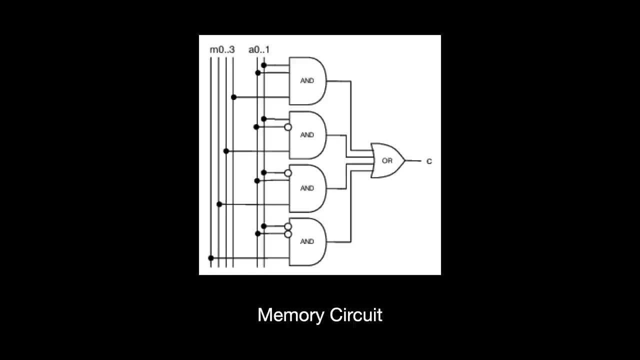 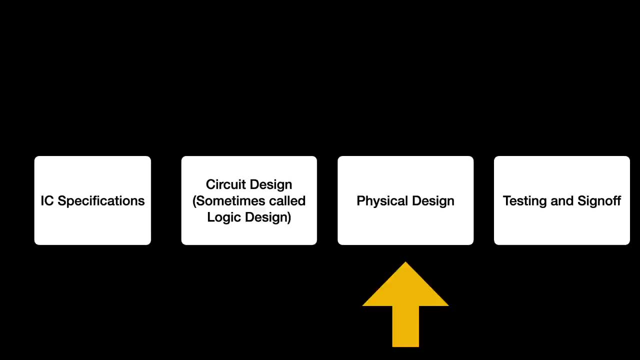 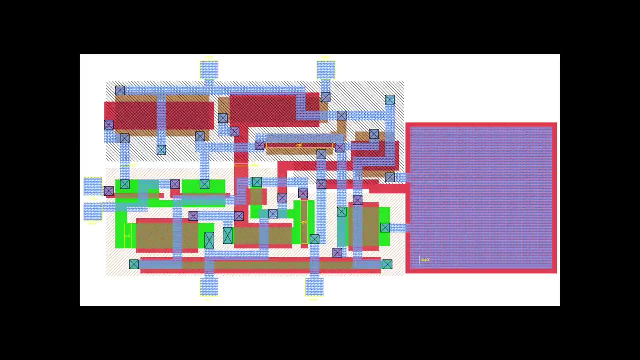 memory circuits connected together with wires. This grouping is referred to as a netlist. After the logic design process, the design gets handed over to the physical designers. The work they do involves the literal, physical layout of the logic circuits, memory circuits and the wiring between them on the chip. When you have thousands. 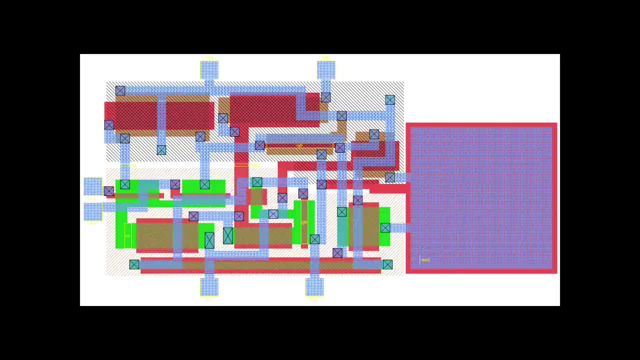 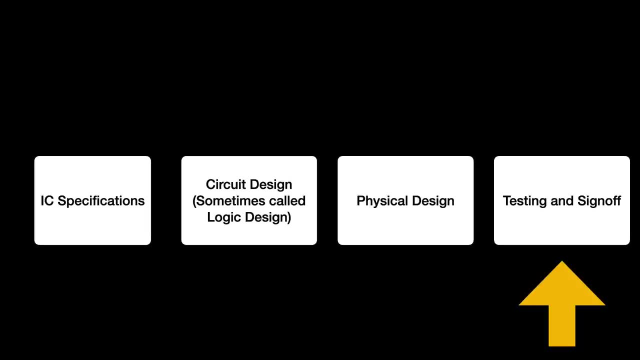 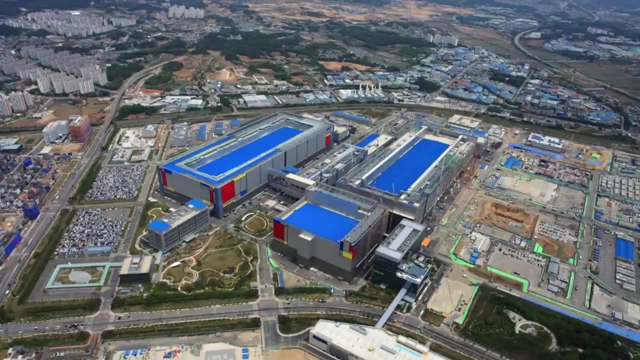 or even millions of such circuits. this can get difficult. Once it goes through all of that, the chip design is verified and tested for errors before being sent to a foundry like TSMC or Samsung Foundry. EDA software is heavily involved in every one of these stages. Even a company like 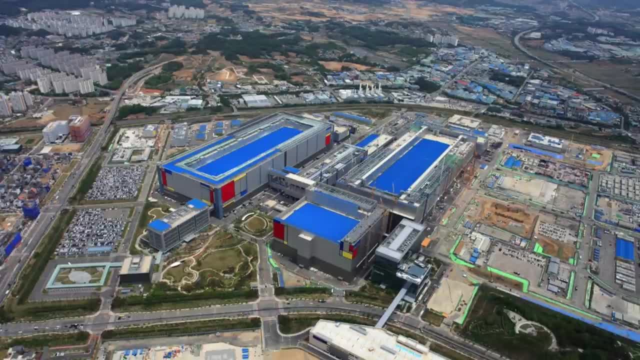 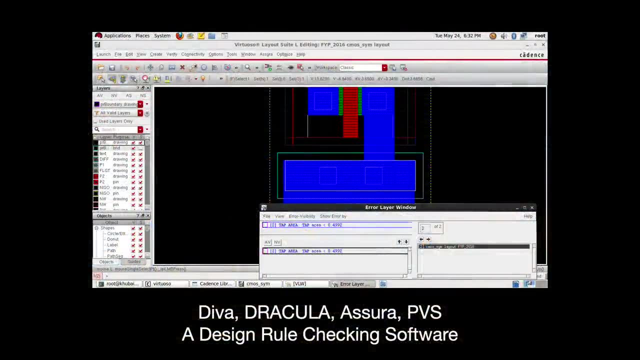 TSMC or Samsung uses EDA software to check a newly arrived design to make sure it is compatible with all of their design rules. Such testing or design rule checking is an especially big deal. An error here can cost millions of dollars if it slips into the fabrication stage. 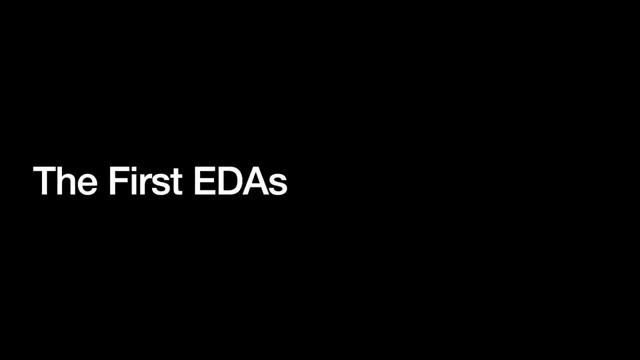 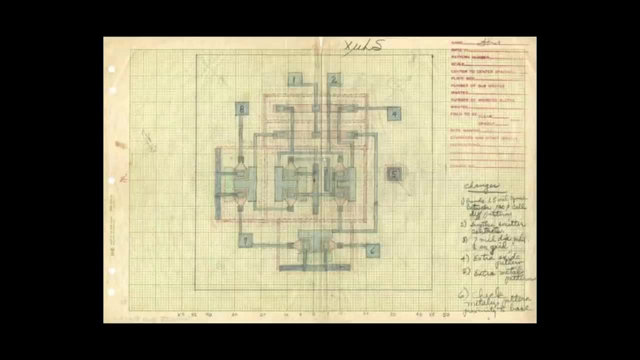 At the early stages of chip design, basically into the 1970s, chip designs were done by hand. The designer would draw a design on paper. This paper design would then be transferred to a photomask made of a material called rubylith. 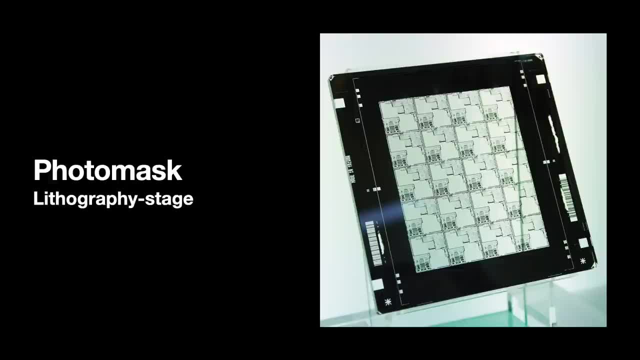 The photomask can then be used to produce the chip design's patterns on the substrate. This is done by projecting light through the mask onto the material And so on. But as chips got increasingly more complex, with more transistors and connections, 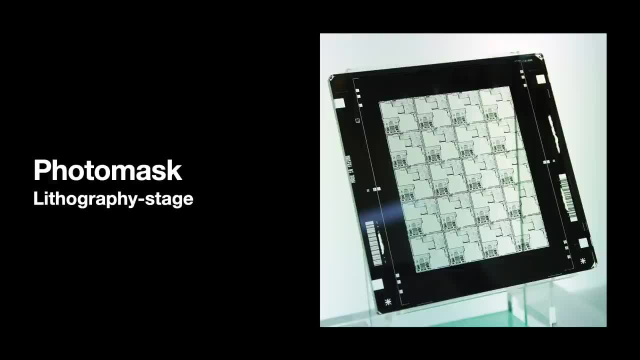 simple software tools were developed in-house by the big companies to aid in the design process. These tools would become the EDA software tools used today. The first software programs automated the placement of a very small number of blocks and wires on a circuit board. 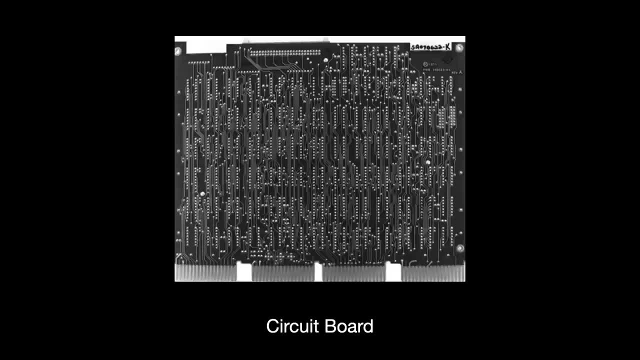 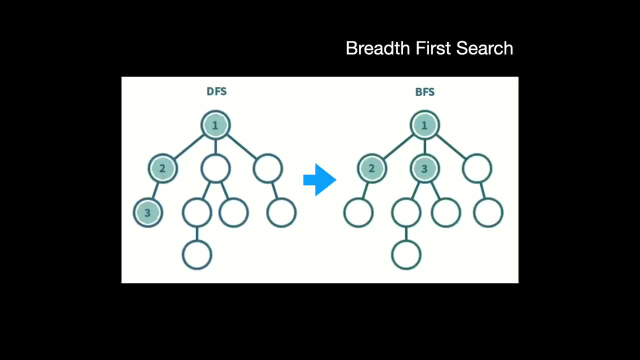 Not a chip But a circuit board. Routing makes sense for these early programs because the task gets tedious. It also needed to be constantly done over and over again as board components moved around. At the beginning these big mainframe programs ran simple breadth-first search algorithms across a grid. 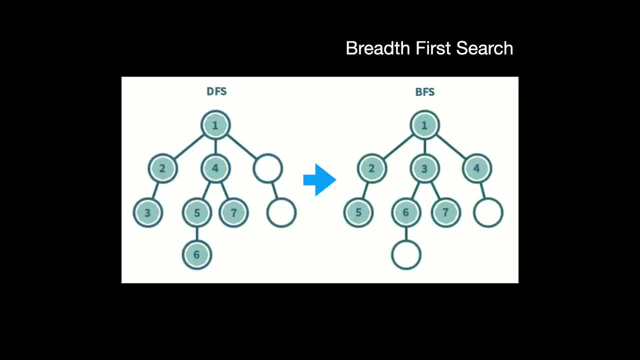 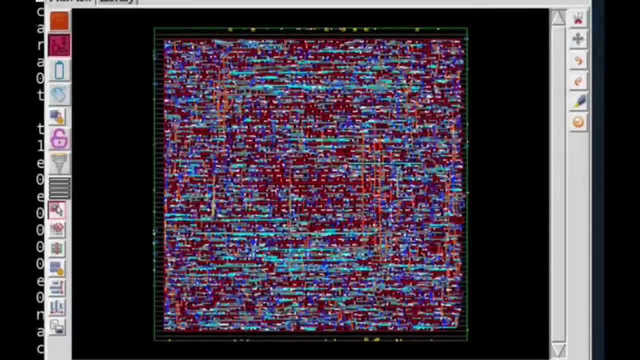 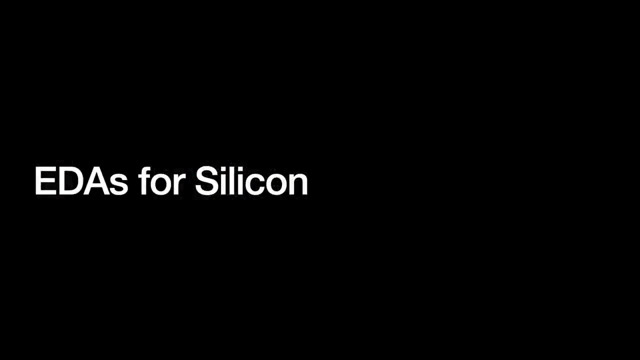 Breadth-first, meaning that they explore all the possibilities at a single level first before diving deeper to the next level. This was rather slow, so these programs quickly moved on to other algorithms in later versions of the software As a number of components within an integrated circuit started to exceed that on a circuit board. 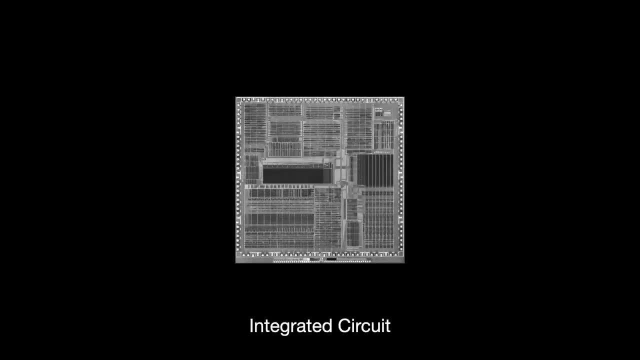 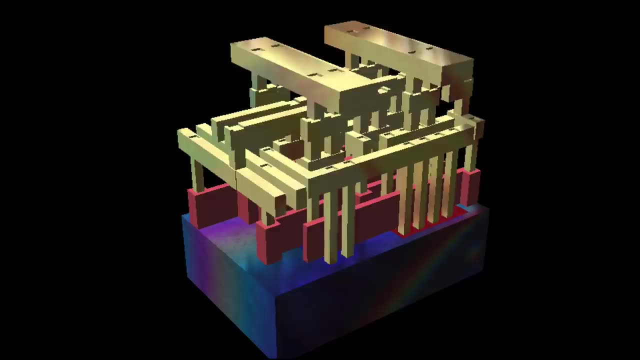 EDA software usage moved to the silicon realm. Bringing EDA to silicon helped solve daunting challenges in chip making. A chip is built in layers. Now you have to wire connections in 3D, taking into consideration layer-to-layer connections called vias. 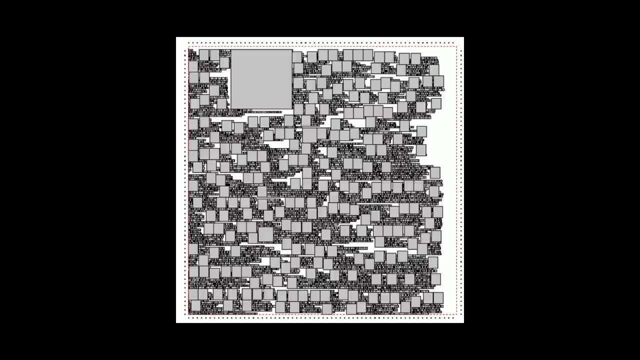 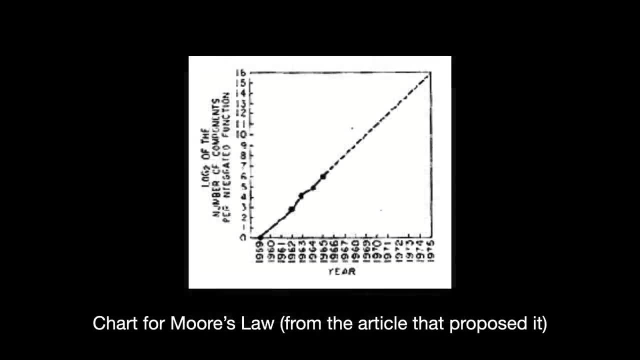 It adds astounding amounts of complexity and presents huge opportunities for errors and would lead to chip design. Moore's law- an observation, not a real law- set the pace for the semiconductor industry to produce chips with ever-increasing numbers of transistors. 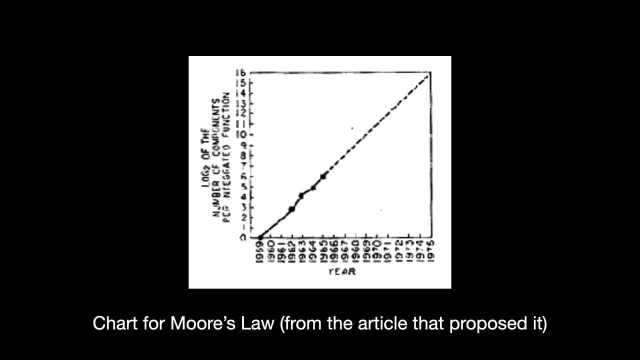 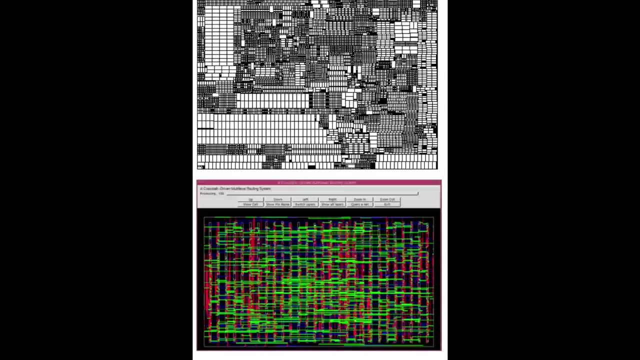 Assuming the industry follows Moore, that translates to roughly a historical 58% annual rise in the number of transistors that fabs are capable of fabbing. Being capable of fabbing that many transistors is one thing, but designing the actual transistors to be fabbed is another matter. 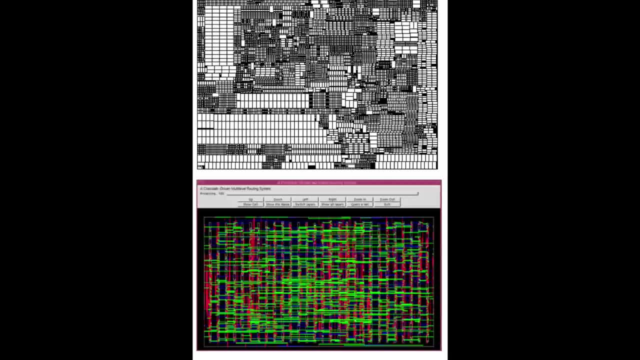 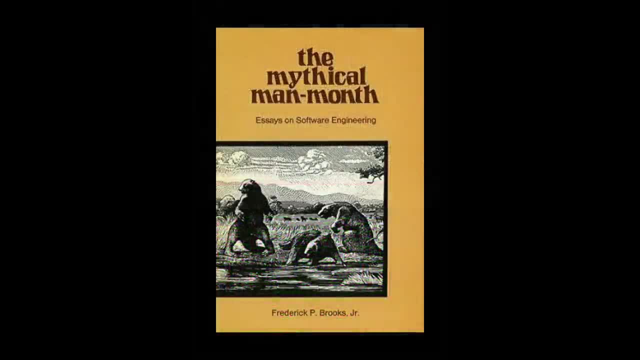 design can only be done in a very few computers. design can only be done in a few computers go along so fast because human knowledge and skills cannot scale up as fast as tools and capital. And if you disagree with that statement, then I recommend you check out The Mythical Man. 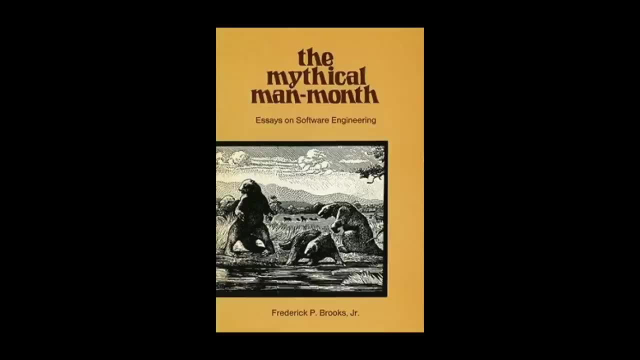 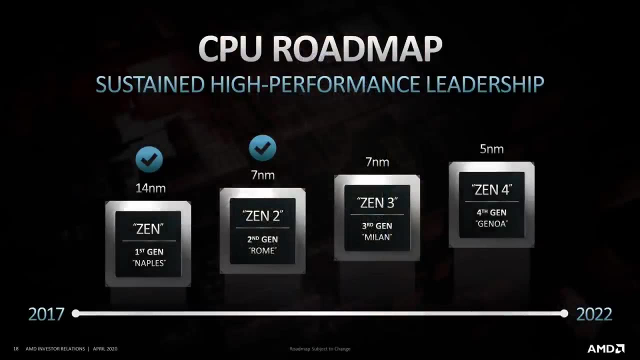 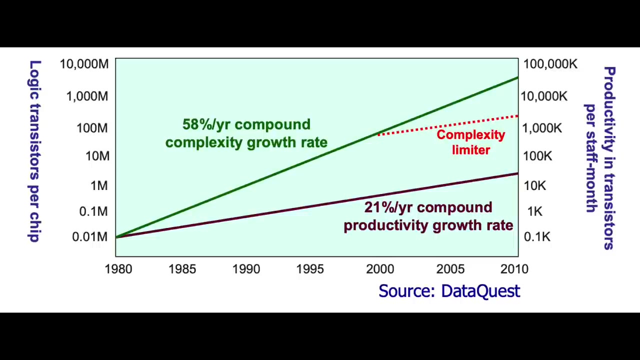 Month or other works on project and software management. At the same time, consumers want that next hot chip in their hands right now. What results is a gap in productivity between design and manufacturing capabilities A company like AMD might need a few years to come out with. 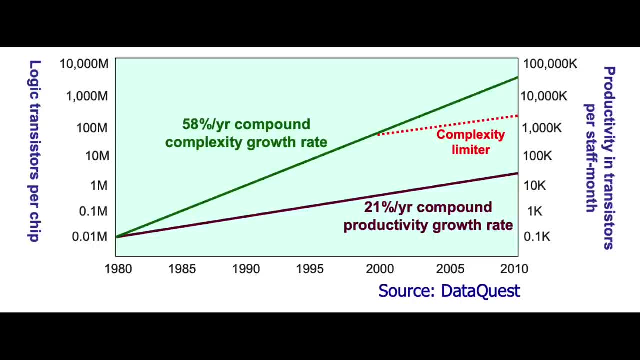 a 5nm chip, even if TSMC had the capacity for them to use. Imagine if mega-customers Apple and Huawei weren't around. Would TSMC even bother to put out a 5nm process node so quickly? Better EDA tools are the only practical way that chip design teams can keep up. 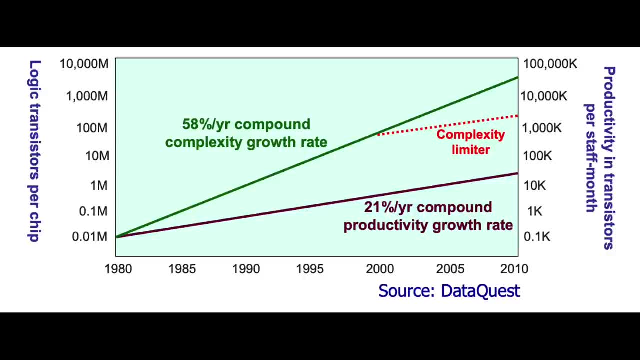 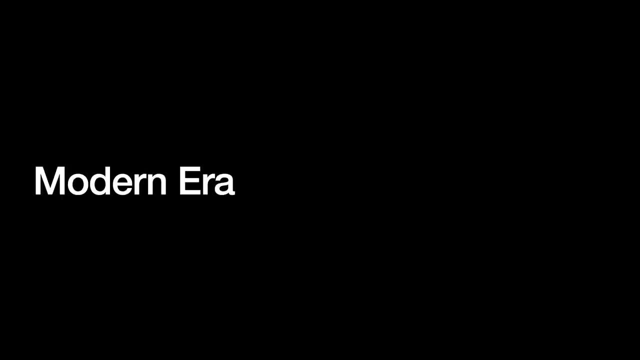 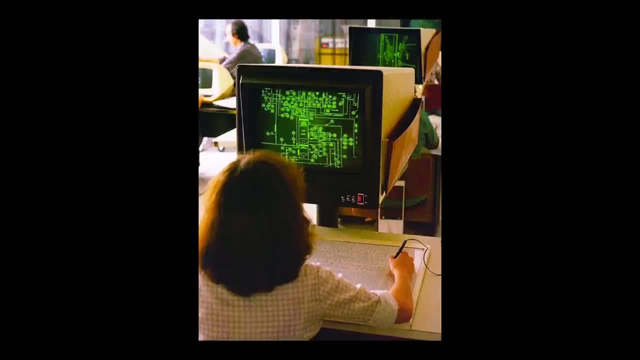 and close the productivity gap. Commercial automatic physical design systems began emerging in the 1980s. They came as a result of not just improved computing capabilities but also improved performance. The first EDA software literally just drew things on paper like a printer. The advent of reasonably 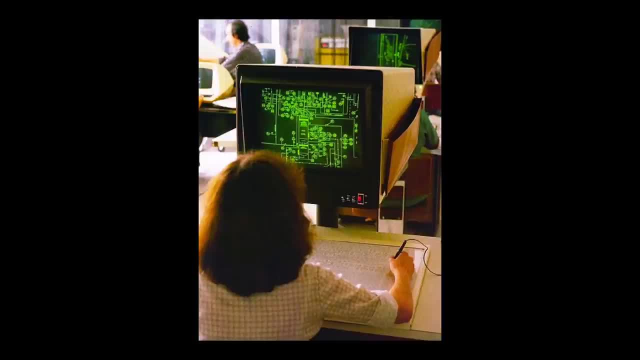 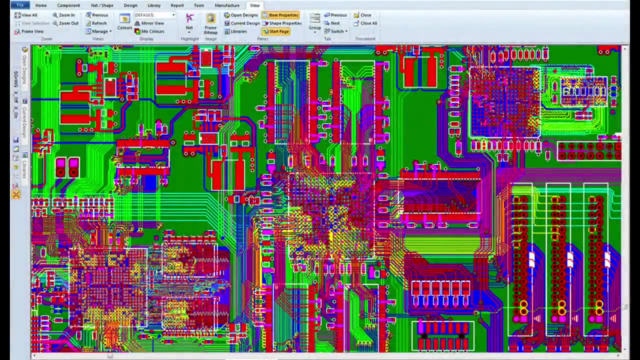 priced storage tube class CRT screens made the industry much more accessible to industry designers. The industry also pioneered and adopted new approaches to chip design that unlocked more of the EDA industry's automation powers. Engineers and universities advocated for a more space-efficient design style on pencil and paper. 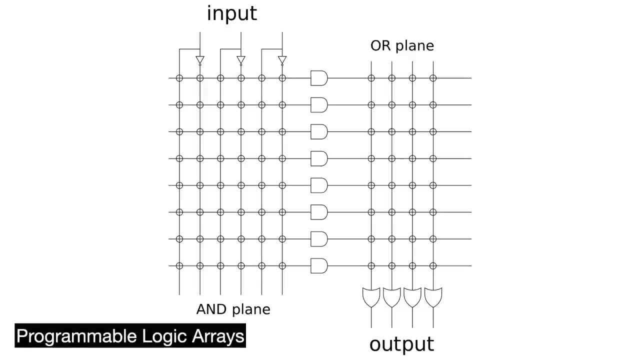 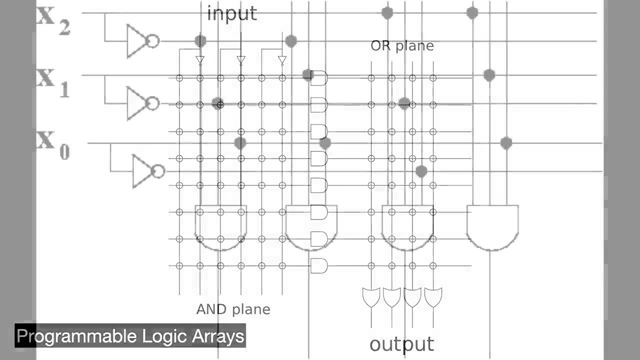 called programmable logic arrays, But EDA software for this style did not scale very well. You had to do a lot of redrawing whenever components changed And conceptually people had to handle the design at both a high and low level of abstraction. 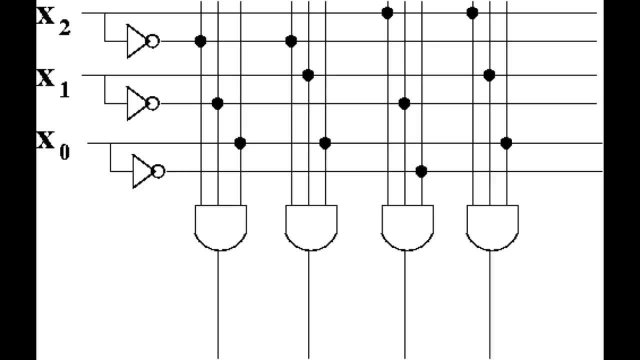 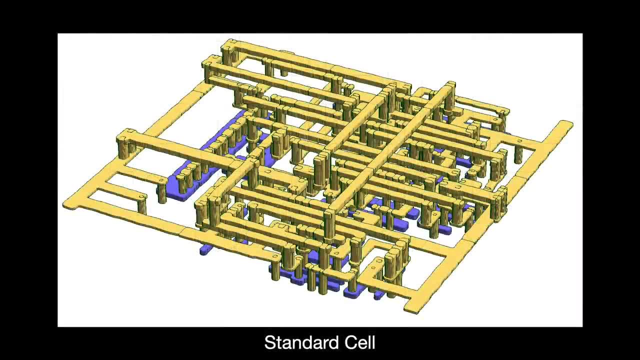 This made design difficult. It is kind of like having to architect a house while crafting the bricks at the same time. The semiconductor industry, on the other hand, developed a standard cell style. Here, designers choose from a library of standard, standardized groups of gates called cells, and decide how they are wired together. 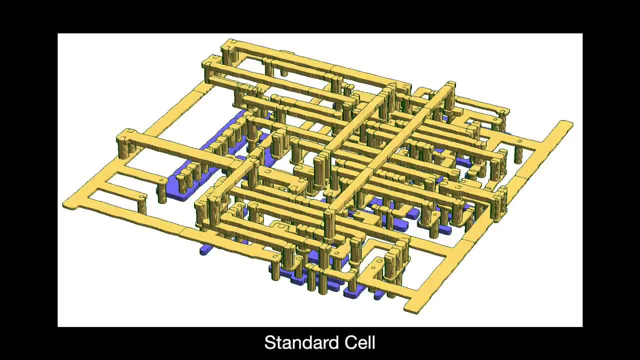 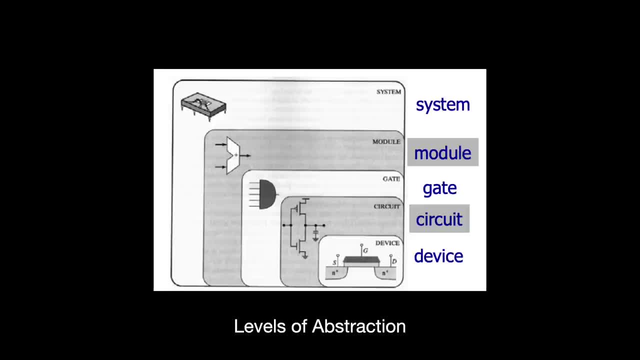 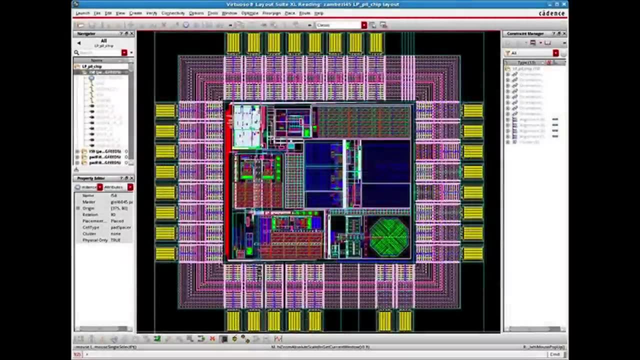 This allowed the design process to split into the separate logical and layout functions I mentioned earlier. It abstracted away the bottom level stuff and let people focus on their own areas. And because the cells are standardized, EDA software can consistently create electrically and physically correct designs all the time. 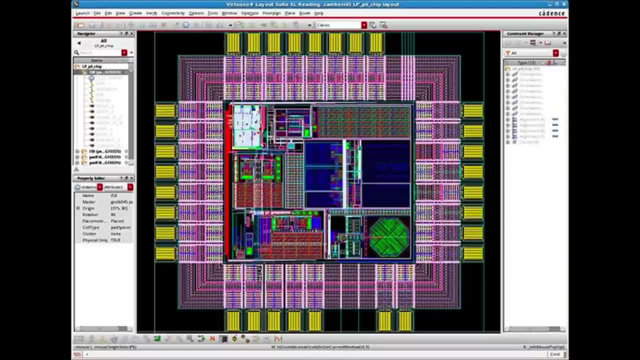 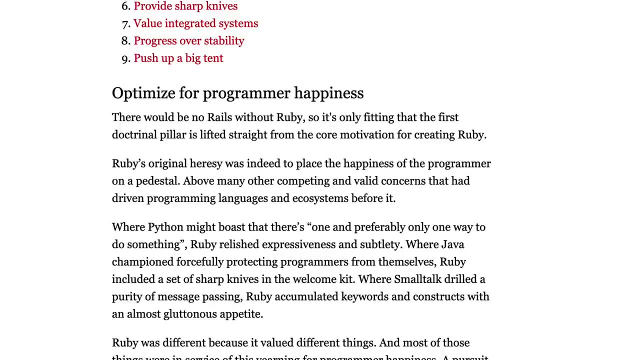 Several people criticized this style for being less area efficient. Some early standard cells had half of their area being taken up by routing. But because its EDA worked so much better for designers' workflow, it became the industry standard. Think of it like with programming: You can write, test and debug a program much faster. 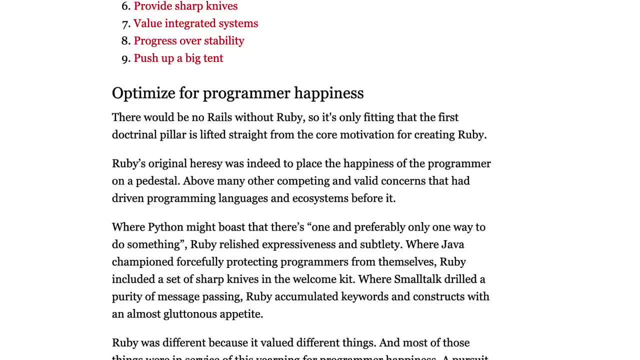 if you did not have to sit and wait several minutes for your code to compile every time you made a change to it. Such a programming language is likely to gain traction, even if it isn't as efficient as other alternatives. An EDA industry sprouted to service various 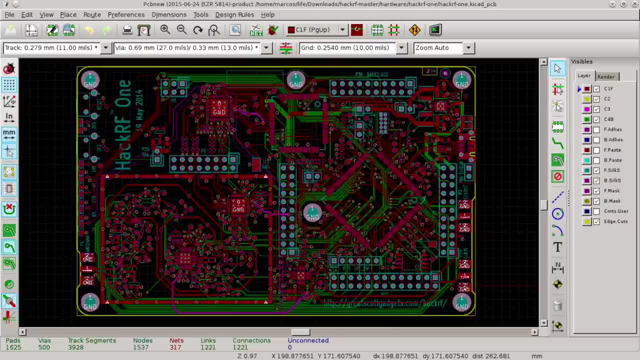 parts of the chip design process, For example, the chip design process for the EDA software. EDA is a central component in the ESA framework. Over time, these software firms consolidated as tasks got harder and required integration across various stages of the design cycle. 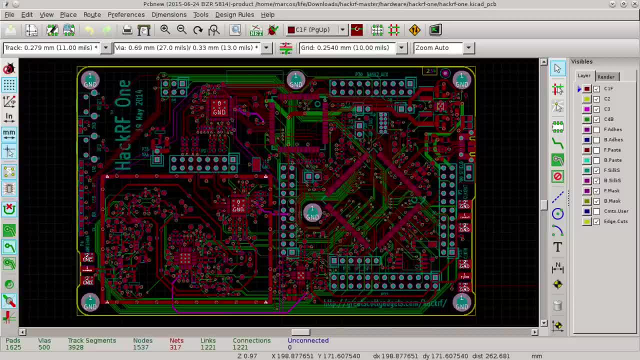 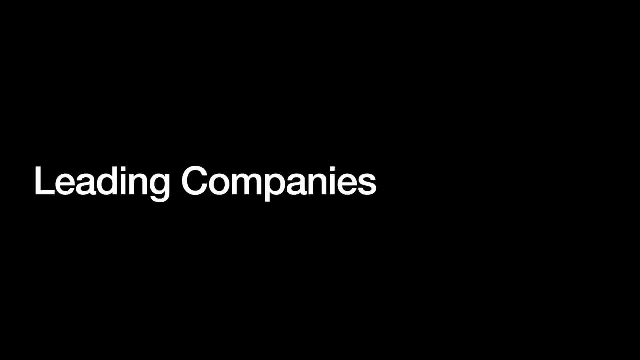 Their proprietary libraries would end up being the de facto standard across the entire industry. The two leading companies in this space are Kadence and Synopsys. Both are based in the United States and are publicly traded. Kadence has a $34 billion market capitalization. Meanwhile, Synopsys is in its 31st year. We are working and working to build this core system to help credit рассurances for such a long time as possible. Before we get into anything new, I needed to know the costs, So took our ganska detailed analysis of all the initiatives and challenges and presented it to the 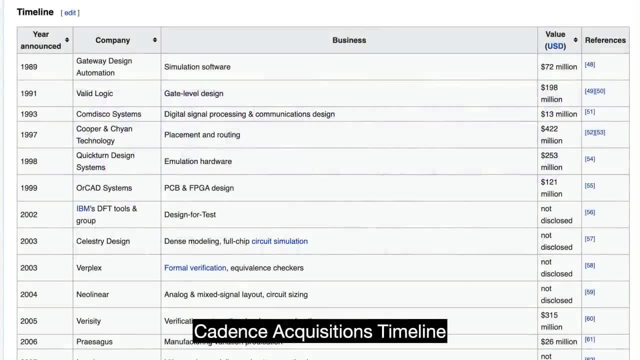 People who expect exciting puzzle research. To slowly get to it, you will need some basic ideas and, before we get involved, make your own measurements and we will eye now what to look as we can make. companies are the creation of a long series of acquisitions They have been involved in. 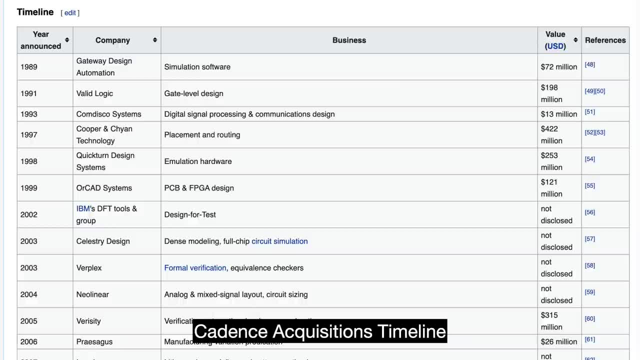 the industry for a long time and have struck alliances with large players like TSMC and Samsung Foundry to help solve problems in transitioning a chip from the design to the real world. They just make things so much easier For fabless entrants looking to enter into the. 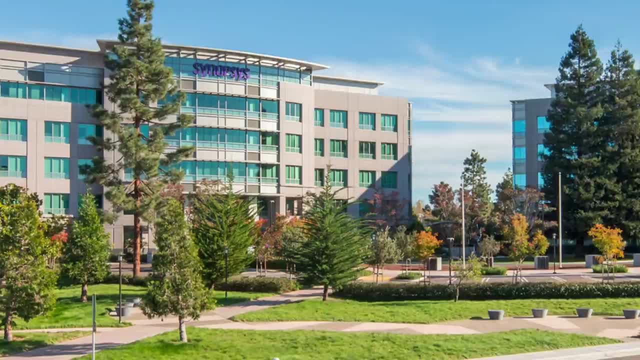 semiconductor world. they likely have to go through these EDA vendors and get their software to get started. Your company might have to pay millions of dollars to acquire a whole bundle of software tools- a common trick in the SaaS world. Beyond just the EDA tools, the companies own a lot. 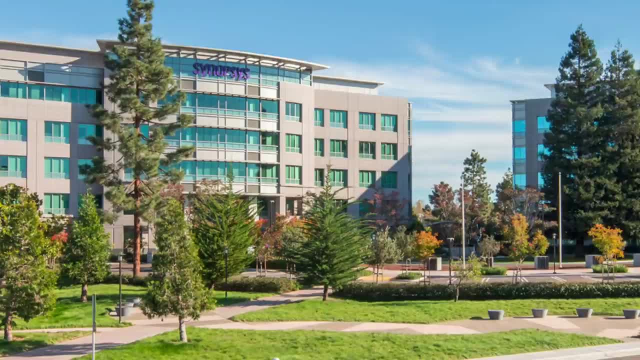 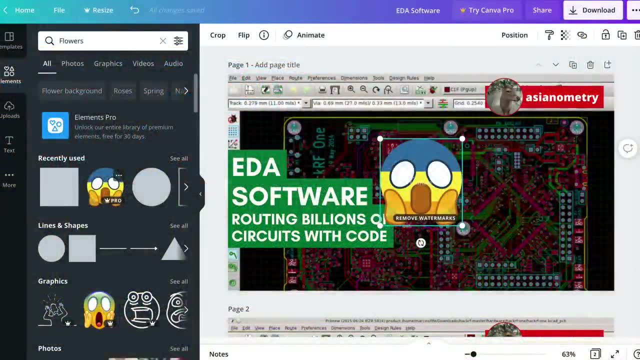 of IP as well. They make money licensing out useful IP blocks for standard functions in a chip like I-O, Kind of like how in Canva, the online graphics design tool that I use to make my videos, you have to pay $1 for this little emoji or flower of clipart that you want to use in your design. 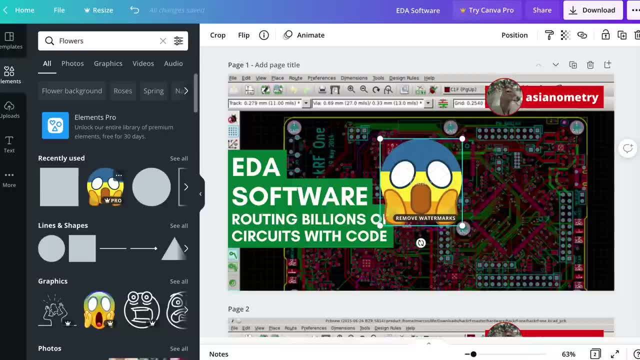 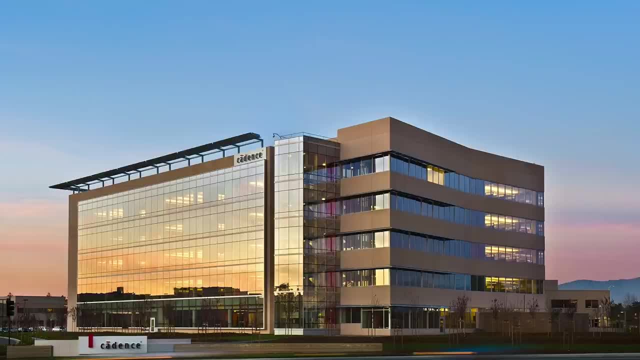 Sure, I can go for something else or even make my own, But why bother? This works the best and is the most convenient. As a result, both companies have very good gross margins and strong cash flows. Software subscriptions and IP license businesses are like that.